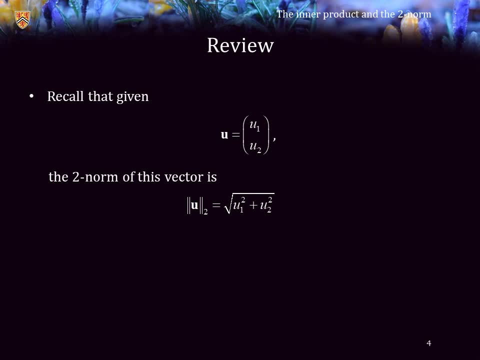 two-norm is just defined as the square root of the sum of the squares of the entries. Thus we will define the two-norm as the square root of the inner product of u with itself. That is, the two-norm is the norm that is induced by the inner product. Now, later on in linear, 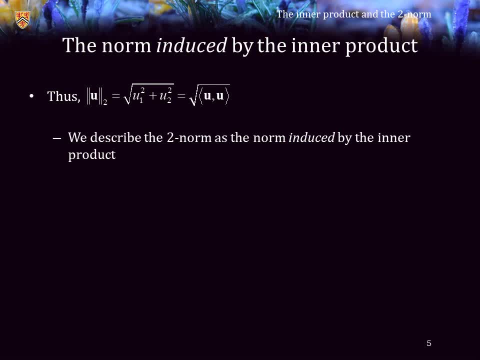 algebra, you're going to see a lot of other norms that are very useful in engineering. however, in those circumstances where we are using the inner product, invariably the two-norm is the most important norm in question. So the two-norm is always going to be defined. 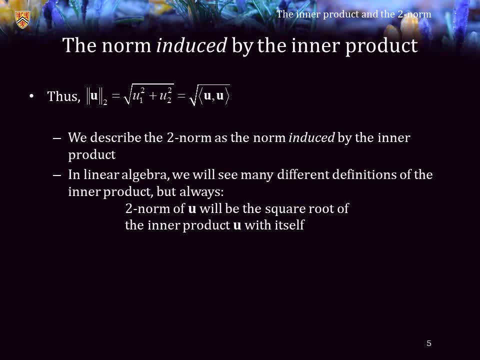 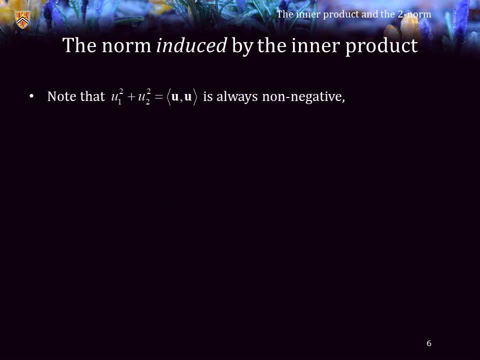 as the square root of the inner product of a vector with itself, and later on we're going to see many other vectors that are not one and two-dimensional but rather n-dimensional, so it's going to be called the infinite-dimensional. Now note that the sum of the squares of 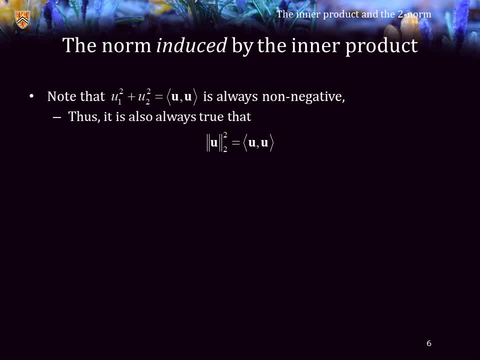 the entries is always non-negative, and thus it is also true that the square of the two-norm is equal to the inner product of u with itself. Also, the inner product of u with itself is equal to zero if, and only if, u is the zero-vector and if, and only if the vector u is a independent vector. 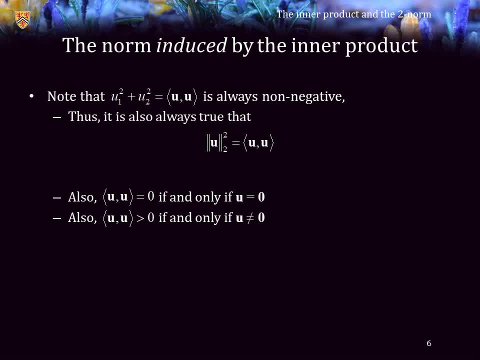 And the inner product must be strictly positive if, and only if, u is not the zero vector. So for every single non-zero vector, the inner product of that vector with itself must give a positive number. Now remember that when we were looking at the 2-norm. 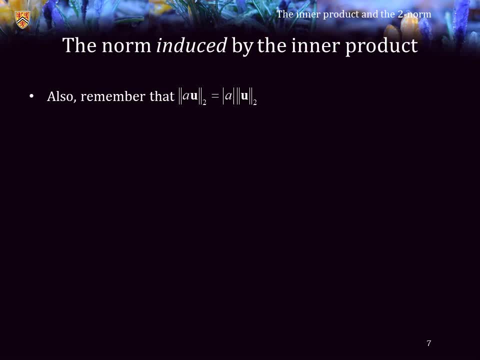 as defined as the sum of the squares of the entries. square-rooted, we saw that the 2-norm of a scalar times u is equal to the absolute value of that scalar times the norm of u. So, for example, if a is equal to 3, then the 2-norm of 3 times u is 3 times the norm of u. 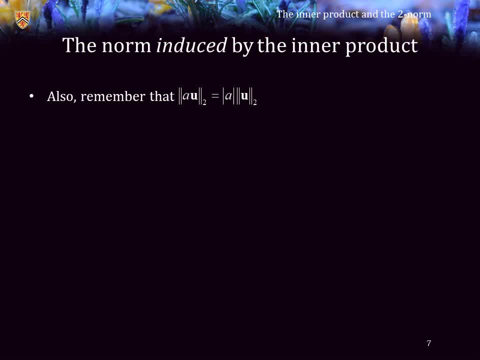 Similarly, the 2-norm of negative 4 times u is the absolute value of negative 4,, which is 4, times the 2-norm of u. Now we deduced this by using the definition of the 2-norm. 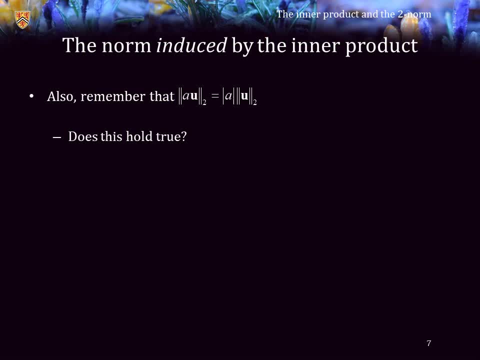 Does it still hold true if we define the 2-norm as the square root of the inner product, with u with itself? Well, recall that if the second entry of the inner product is multiplied by a scalar, we can just take that scalar out. 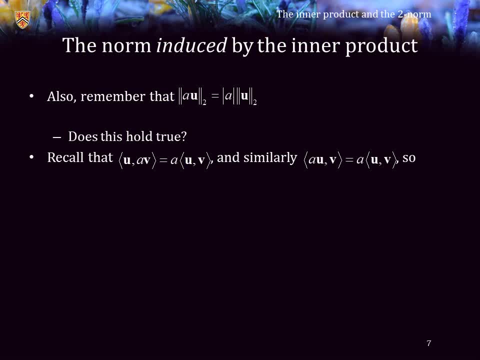 Similarly, because the inner product is symmetric, if the first entry is multiplied by a scalar, we can similarly take that scalar out. Thus, consequently, if we take the inner product of a times u with itself a times u, well, first we can take out the scalar from the first entry. 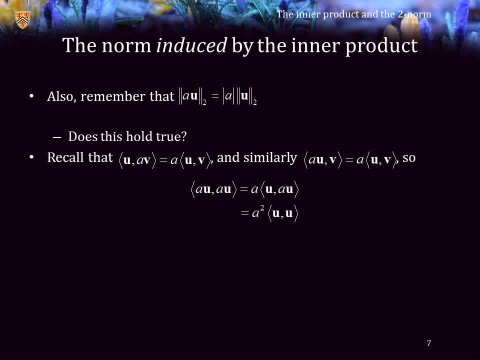 and then we can take out the scalar from the second entry. Now, a squared is greater than or equal to 0,. the inner product of u with itself is greater than or equal to 0,. the inner product of u with itself is greater than or equal to 0,. 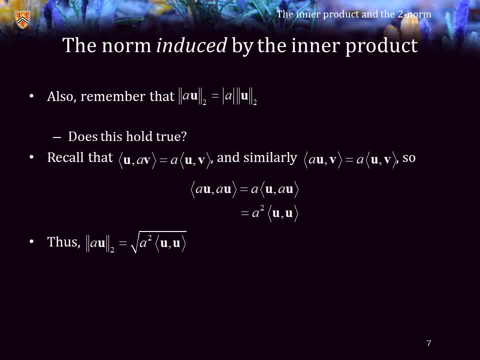 and if we defined the 2-norm of a times u as the square root of the inner product with au and itself, then this equals the square root of a squared times the inner product of u and itself. But a squared is positive and therefore we can separate the square roots. 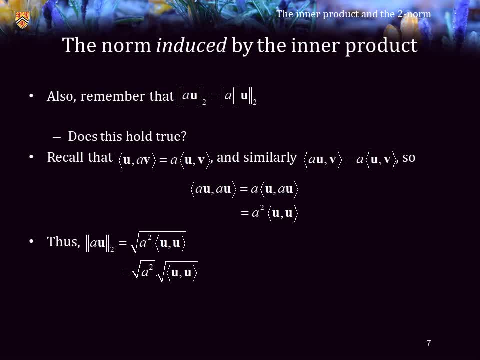 But the square root of a squared is greater than or equal to 0,. the inner product of a squared is just the absolute value of a, and the square root of the inner product of u in itself is just the 2-norm of u as we define it here. 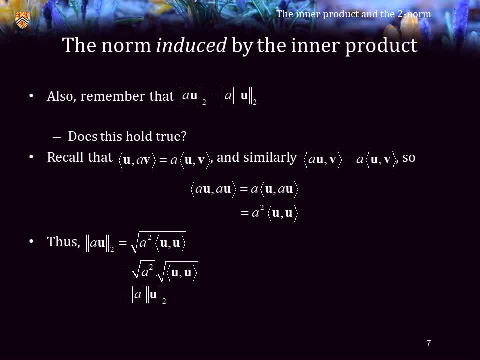 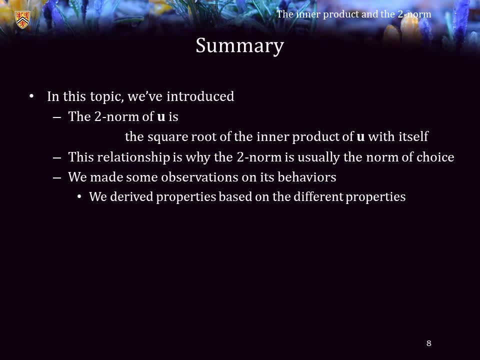 Thus this must also continue to hold to be true. Thus, in this topic, we have now introduced that the two-norm of u is defined as the square root of the inner product of u with itself. This relationship is why the two norm is usually the norm of choice. 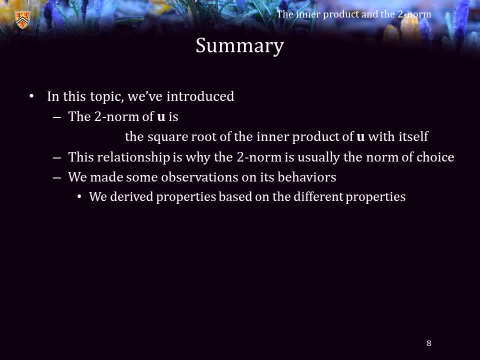 In certain specific applications of vectors. there will be other norms we will use, But if we are using the inner product, invariably we will be using the two norm. We made some observations on its properties and we were able to derive properties based on the properties of the inner product. 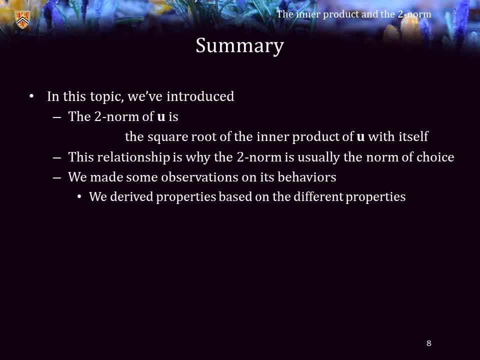 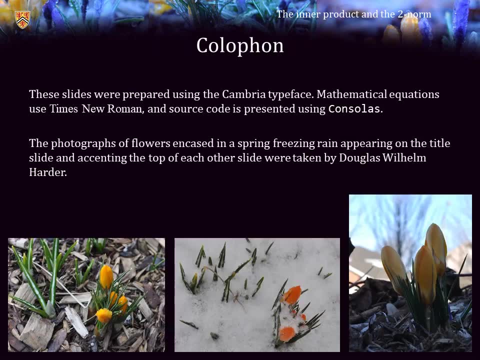 as opposed to previously, the properties of the definition of the two norm. Here are some references, acknowledgements, the colophon and a disclaimer. Cheers.